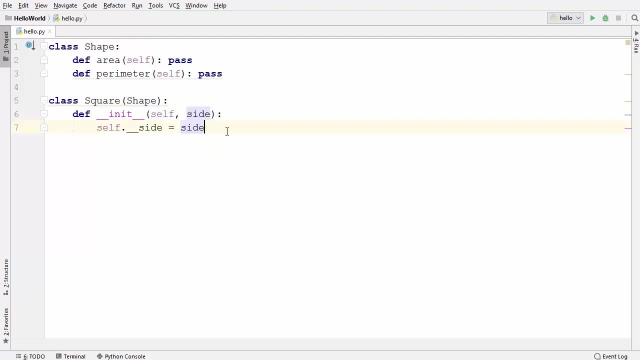 Now, in this example, I want to do two things. One is, I don't want to allow the other users to create an instance of a shape class, Because shape class acts like a template for the square class. So I don't want to allow the users to create an instance of this shape class. So let's see right now if we can create an instance of this shape class or not. So I am going to just write. 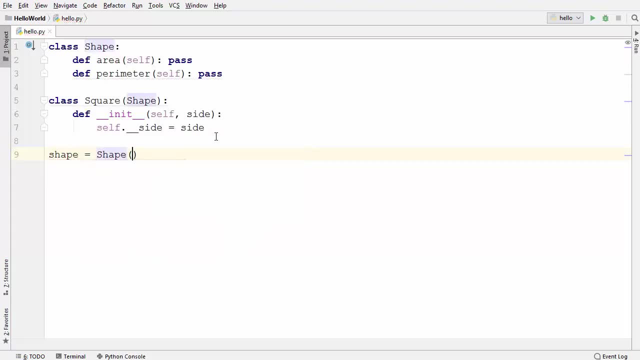 shape is equal to shape and when I run the code, my code runs fine. That means right now I am able to create an instance of the shape class, which I don't want. The second thing is, I want to make sure that both these methods, which are there inside the shape class, are implemented inside the square class. So I want to make sure that whoever is using the shape class, 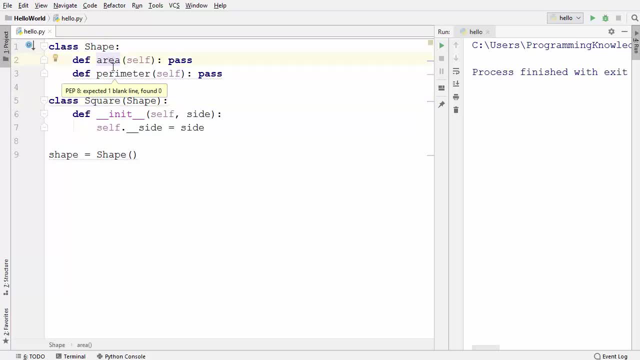 he or she must implement these two methods inside the sub class. So how can I achieve these two things? Now it turns out that abstract classes are just made for that. So how to create an abstract class in Python? The fact is, Python on its own doesn't provide any abstract class, But don't worry, there is a built in module in Python which we can use to create an abstract class. 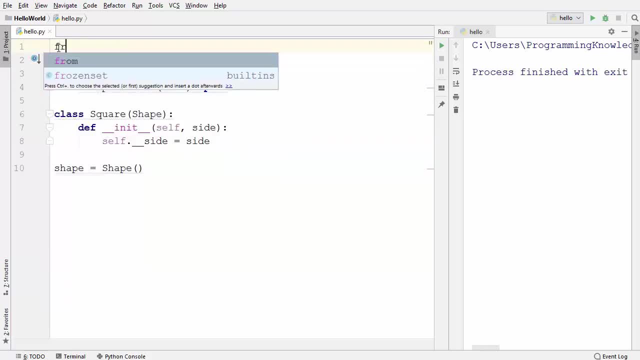 So let's import this built in module first. So I'm going to just write from ABC: import capital, ABC, comma, abstract method. So these are the two things we need to import from this module. Now this module, ABC stands for abstract base classes, and this allows us to create the abstract classes. So how we can create an abstract class using this ABC module. 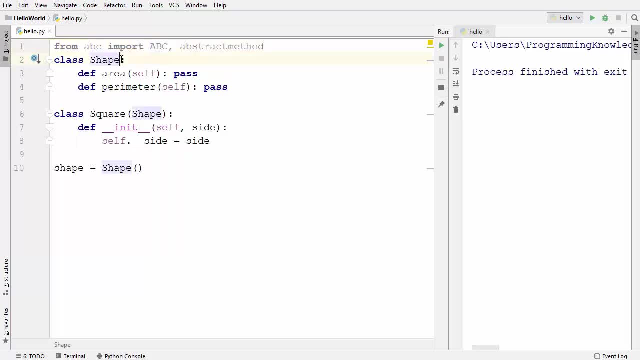 So what we need to do here is we need to inherit from the ABC module into the shape class. Okay, So shape class is inheriting from the ABC module Once this shape class inherit from the ABC module. The second thing what we need to do here is we need to add a decorator here. And how to add a decorator: We just need to use at the rate and then the name of the decorator. 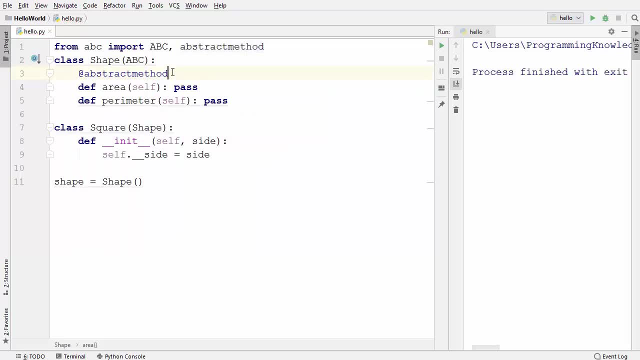 this abstract method which is like this- and let me use this abstract method decorator on top of this parameter method also. so what this abstract method decorator does is it makes these two methods abstract. and what is an abstract method? an abstract method is a method which you must implement in the subclass, so when you run the code now, it will give. 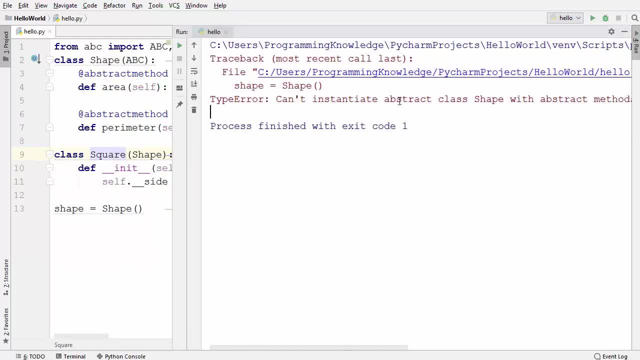 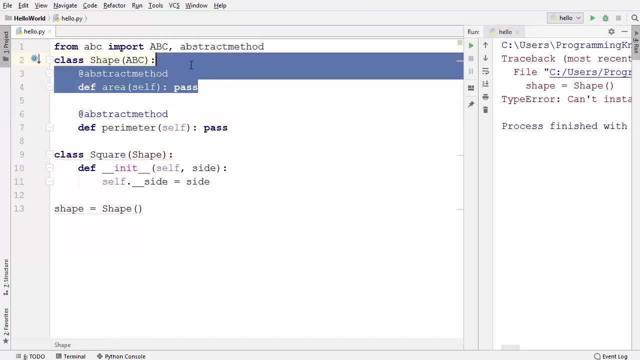 us this error which says: can't instantiate abstract class shape with the abstract method. so once you create any of your class method as abstract, then your class becomes the effect class and then you cannot instantiate this class like this. so our first goal is achieved: that we cannot instantiate this shape class now, because this class is now an abstract. 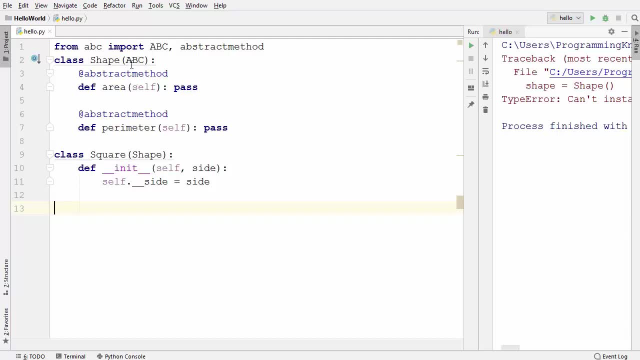 class, and then we cannot create the abstract class like that. so now we cannot create the. and how to create an abstract class? you just need to import the ABC module and then you just need to add this decorator on top of your method. and if you do this, 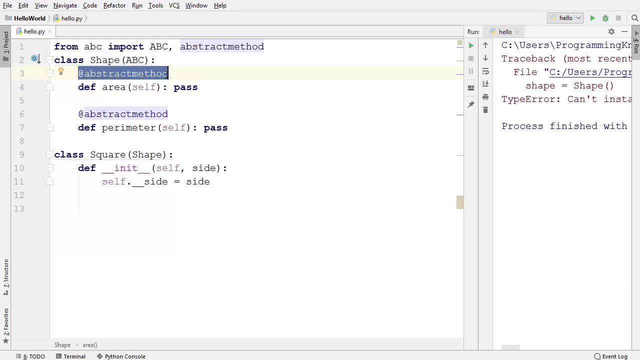 even with one method in your class, then your class becomes abstract. so now we have removed the instantiation of this shape class. but now when I try to instantiate this square object from the square class, let's see what happens. so this square class takes one argument, which is the side of the square, and let 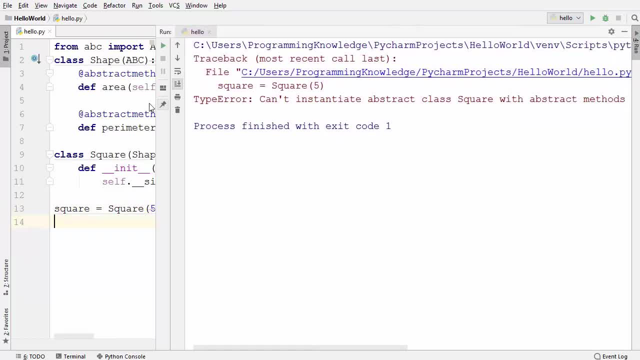 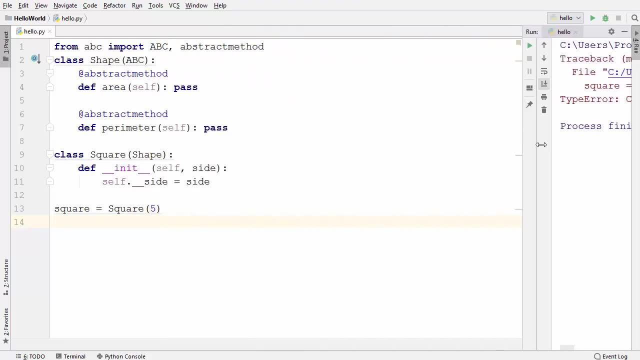 me run this code and once again it gives us an error. and this error says: can't instantiate abstract class square with abstract method. so that means that whenever you inherit from a class which is an abstract class and if this class contain any abstract methods, then the sub class have to implement the methods. 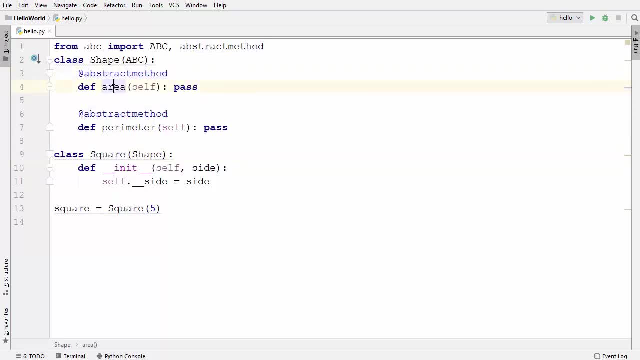 which are abstract. so this method area is an abstract method and this method parameter is also an abstract method. that means we have to provide the implementation of these two method inside our subclass. so i'm going to provide the implementation of area first of all into the 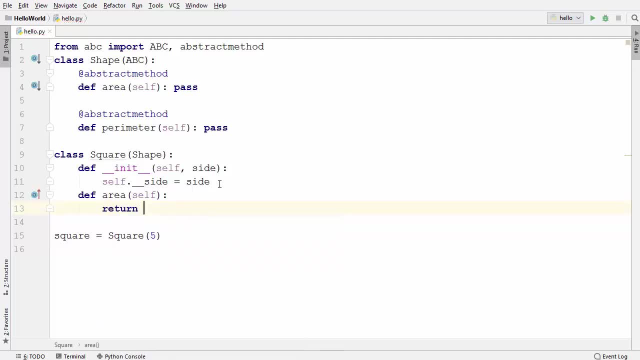 subclass and area. i'm going to just return as the multiplication of the sides, right. so self dot, underscore, underscore side, multiplied by itself. so self dot, underscore, underscore side. and let's say, for now i will remove this abstract decorator from the parameter method and let's run. 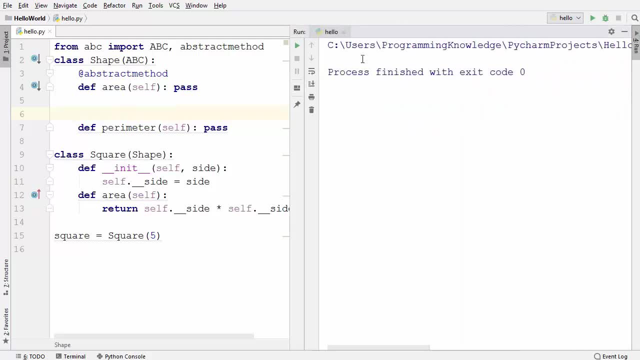 the code once again and you can see it runs fine. so there is no error when we instantiate this class, when we implement all the abstract method into your subclass. so right now there is only one abstract method and we are going to implement all the abstract method into our subclass. so 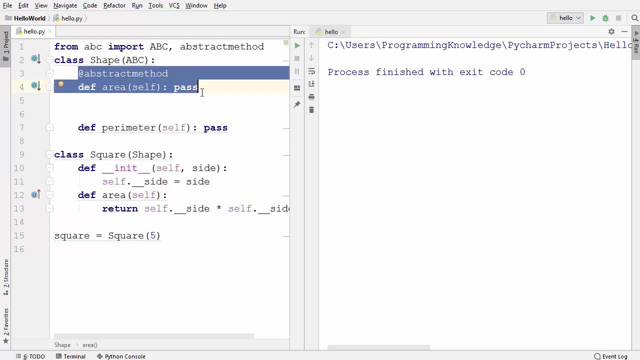 we are going to implement the abstract method, which is area, into the shape class which we need to implement in the subclass, and that we have done so. we see no error here. now let's add this decorator abstract method on top of this parameter method. also, and once again, when i run the code, it: 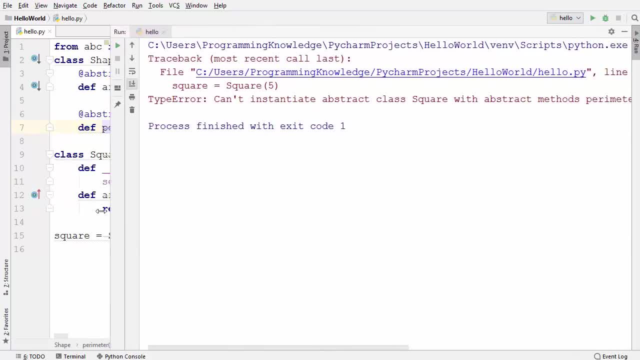 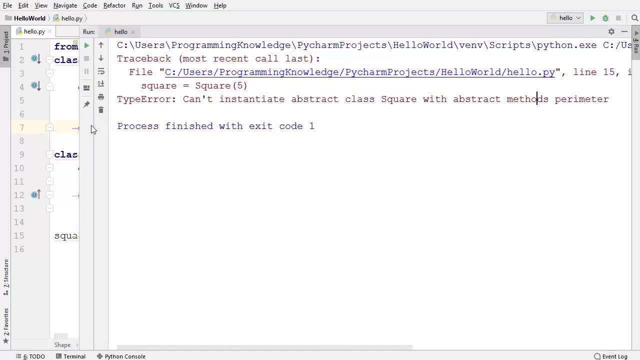 will give me once again this error, and it's going to give me the same error which says can't instantiate the abstract class square with the abstract method perimeter. so we also need now to implement the same error which says can't instantiate the abstract class square with the 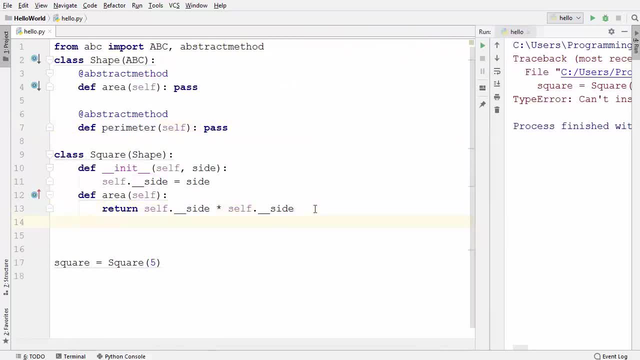 abstract method: perimeter. so let's just implement this parameter method inside the subclass once again. and what is the perimeter? it's four times the size of your square. so self dot, underscore, underscore size. and now we have implemented both of them. and once again, when we run the code, it runs fine. let's also try to print the area and parameter of the square. so i'm going to just print the area of the square. so i'm going to just copy this parameter here from the left inside the came over and paste all the parameters for these pairs, as happened in the manual document. so let's see what happens later on. uh, every utilizing this demo- and we have a- 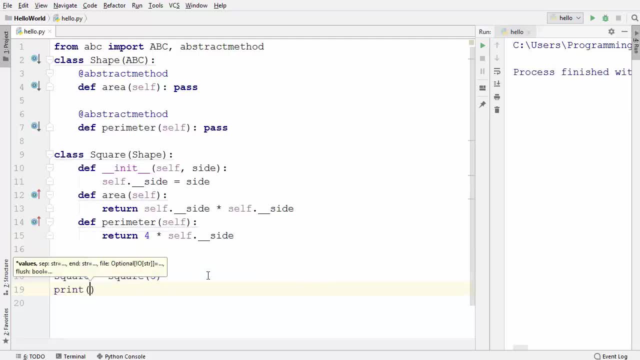 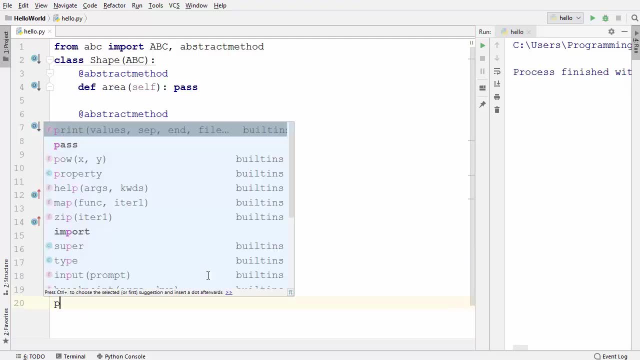 also try to print the area and parameter of the square. so I'm going to just use this object to call the area method and in the next line I'm going to just use print to once again call this object, and this time I will call the perimeter.